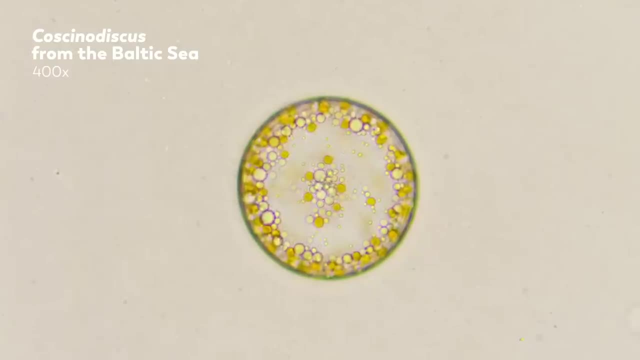 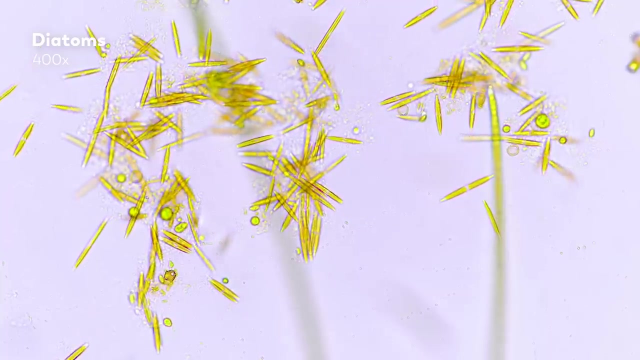 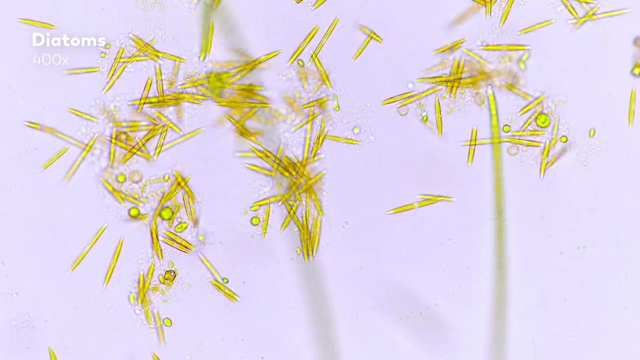 Looking at them through a microscope, you might understand why microbe hunters are so fond of them. They have been called the jewels of the sea. Those beautiful outer shells are called frustules, and they set diatoms apart from every other living creature. 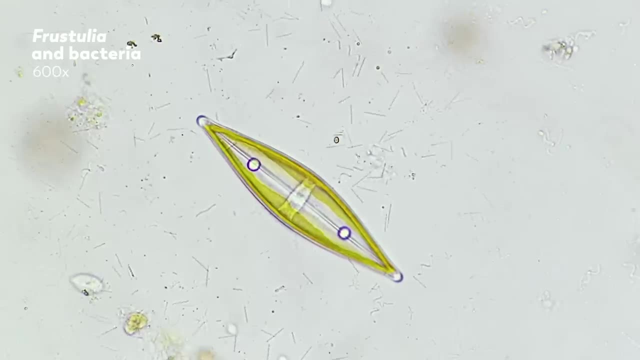 Unlike the organic cell walls and membranes we have seen in the past, the diatoms are a bit more like a muscle structure. If you don't know what the diatom is, you can just call it a cell. In the primary cell cells, the diatom is a cell that is made by some kind of an organic. 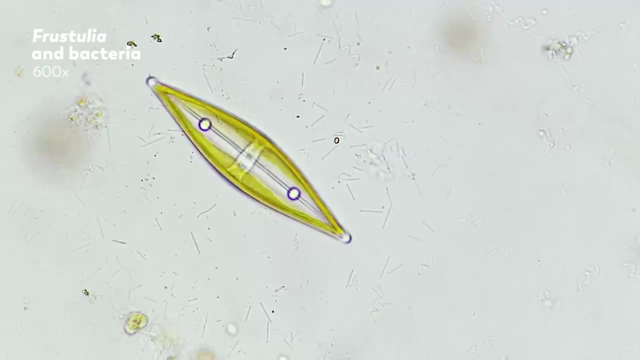 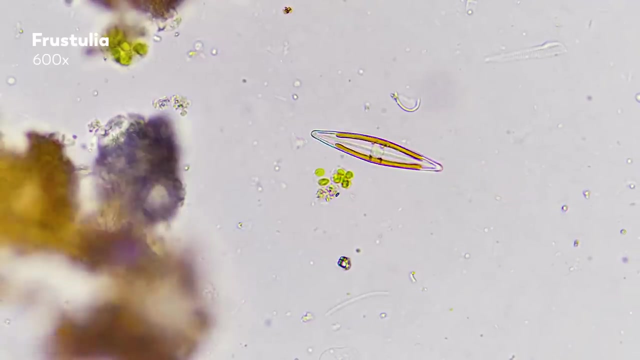 cell. The first cell cell is the cell that we associate with most cells. Frustules are made out of inorganic silica, enclosing the cytoplasm of the diatom in what is basically glass. Silica shells take less energy to make and maintain compared to their organic counterparts. 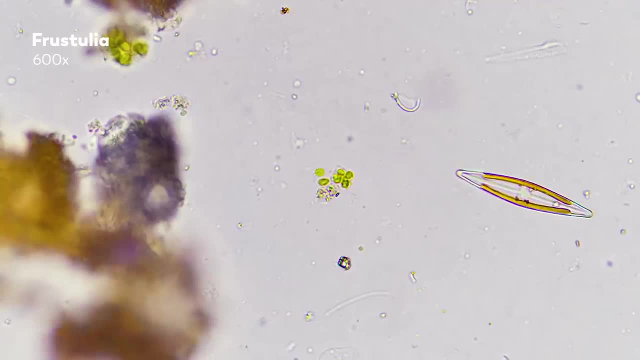 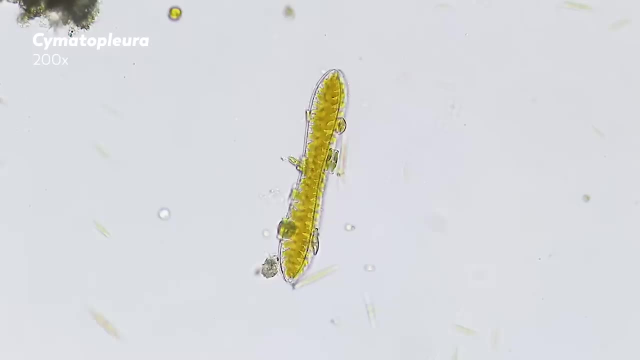 but they do come with a trade-off. Glass is… well, it's glass. It's hard to expand if you're a unicellular organism, organism trying to undergo asexual mitosis, when your cell is enclosed in a rigid, inorganic material. 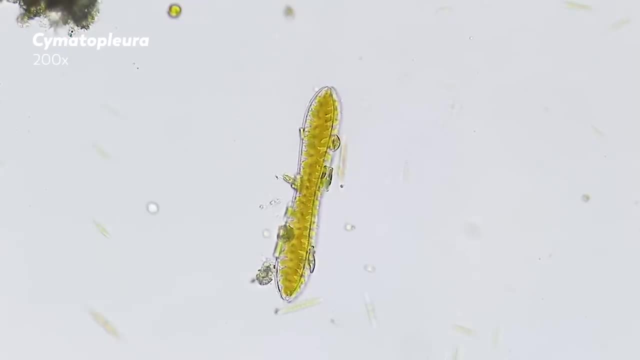 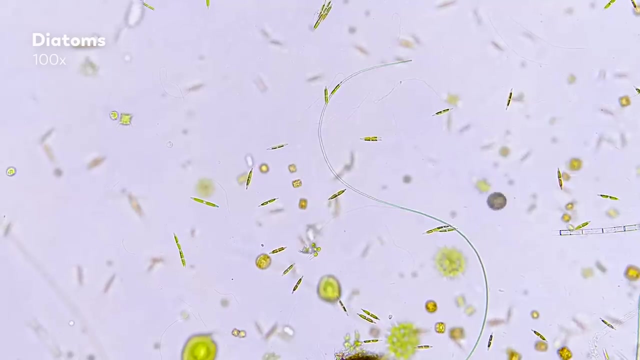 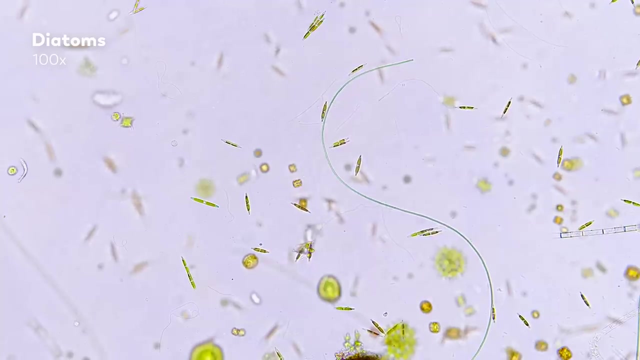 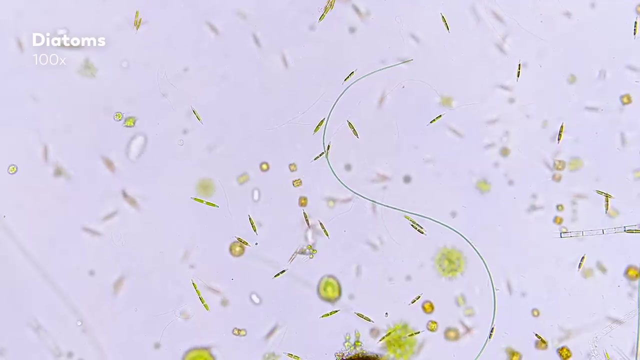 Instead, when diatoms divide the daughter cells, take the old frustule and divide it between them, which means that the daughter cells are both going to be smaller than their parent and they are never going to grow any bigger. And as diatoms keep dividing, the daughter cells keep getting smaller and smaller. 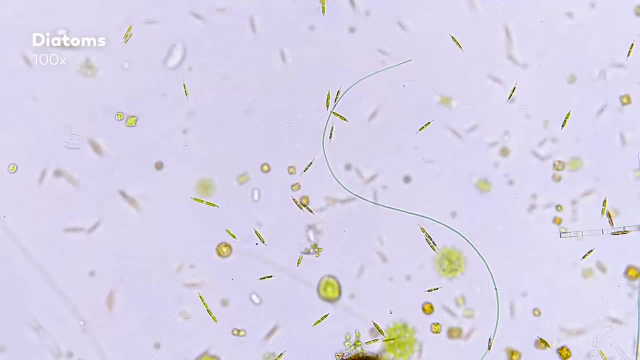 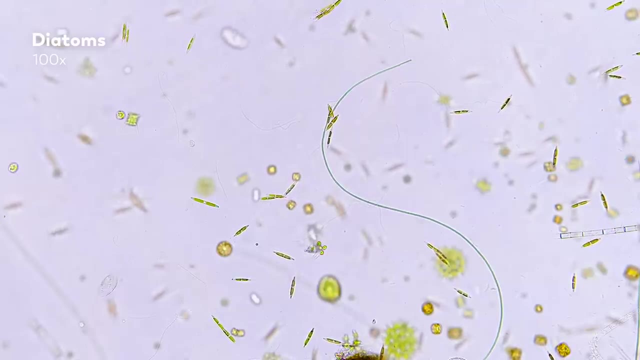 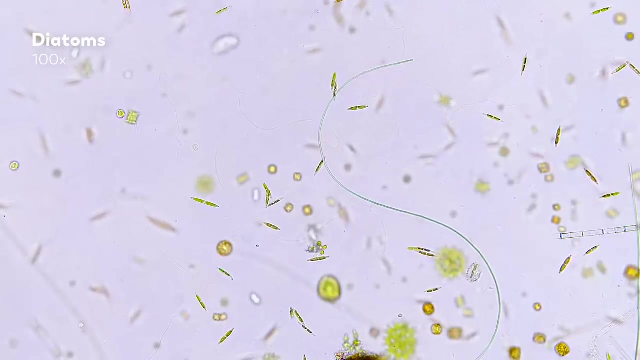 If this goes on forever, the diatom will get so small that it cannot survive. But diatoms that are starting to get too small can avoid that fate through sexual reproduction, which is a kind of refresh button that lets them construct a new frustule for a larger. 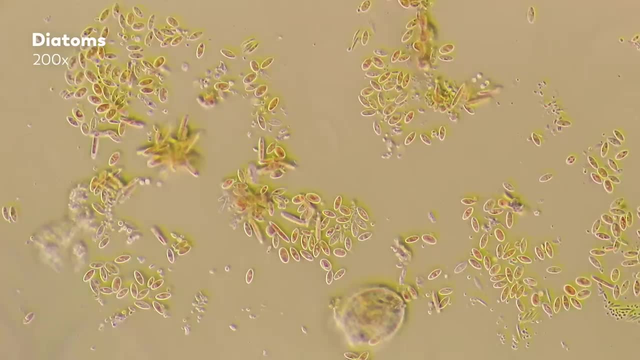 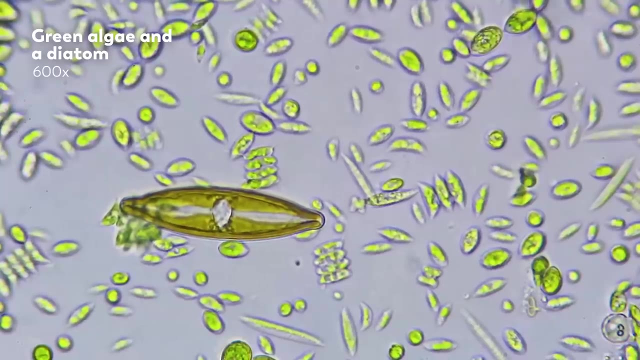 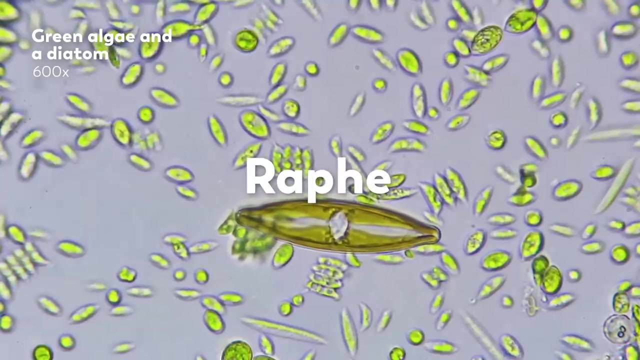 daughter cell. For the most part, diatoms can't actually move. They just go wherever the water takes them. But some diatoms are able to glide along a surface using a slit in their frustule called a wraith. This allows them to secrete mucus that sticks to a surface. 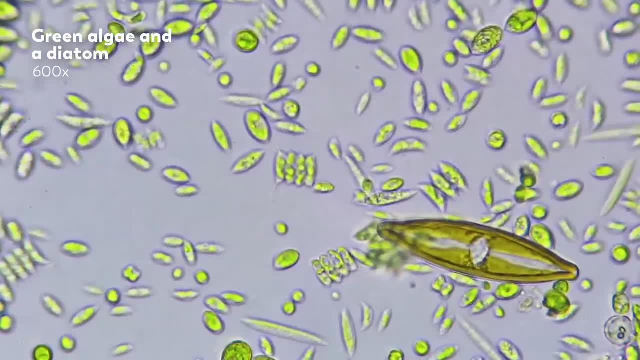 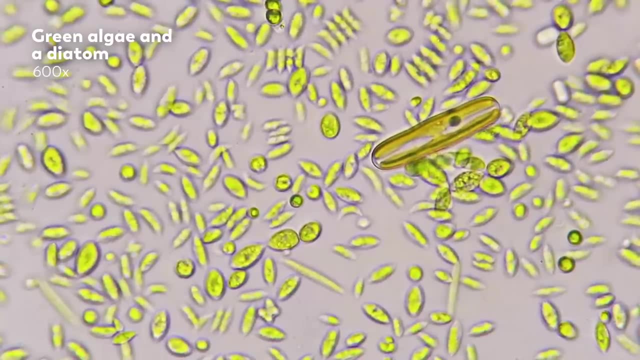 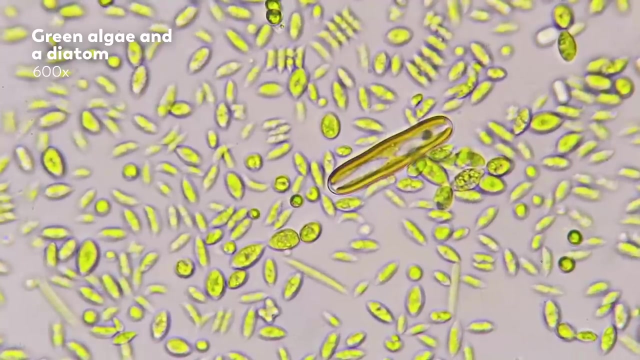 But how does that mucus help them move? We don't know. We can see that they move, So they must be able to, And we can see that mucus is always left behind when they do it, But we don't know the exact mechanism of how it works. 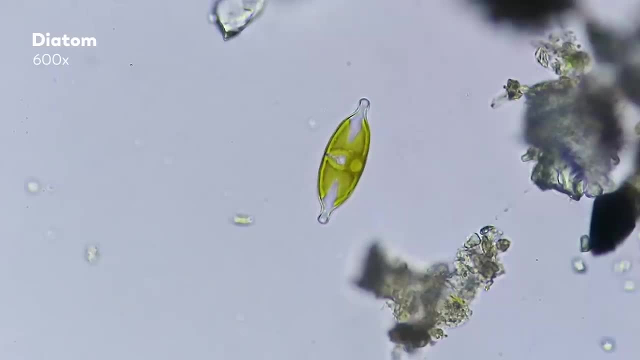 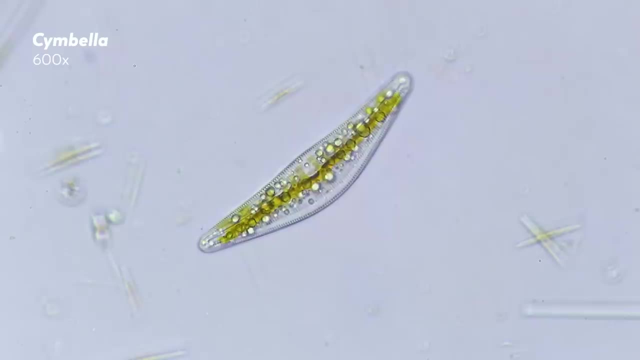 You and I, of course, move using muscles, And the molecules responsible for that in us are actin and myosin. Here's a wild thing: In 1999, some scientists put actin-disrupting compounds in solution with diatoms, and those 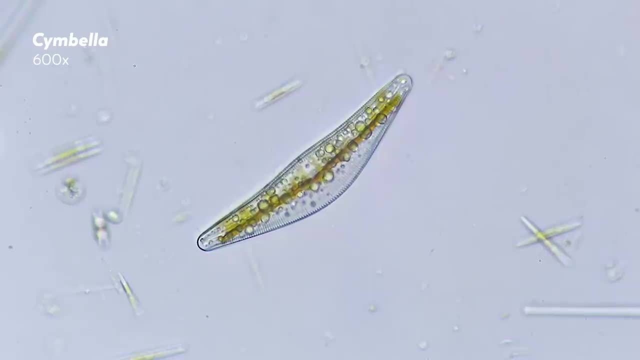 diatoms lost their ability to move, So we can see that mucus is always left behind when they do it. Here's a wild thing. In 1999, some scientists put actin-disrupting compounds in solution with diatoms, and those 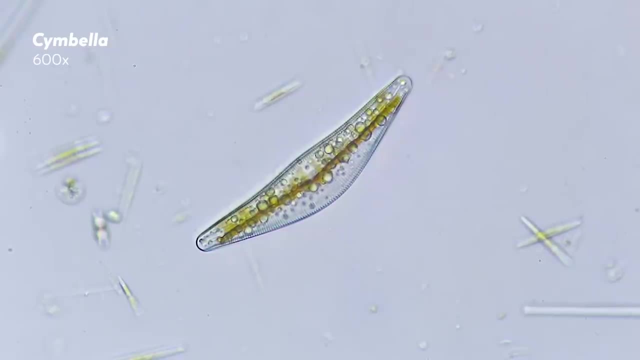 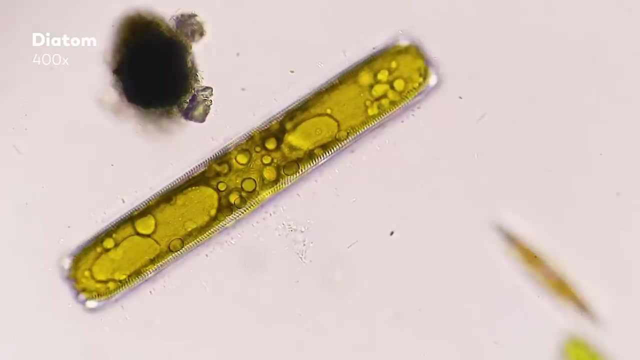 diatoms lost their ability to move, So, while diatom motility remains something of a mystery, these tiny jewel-encrusted algae move using the same molecular systems as us. If you've been looking closely, you might be wondering what these bubbles are. 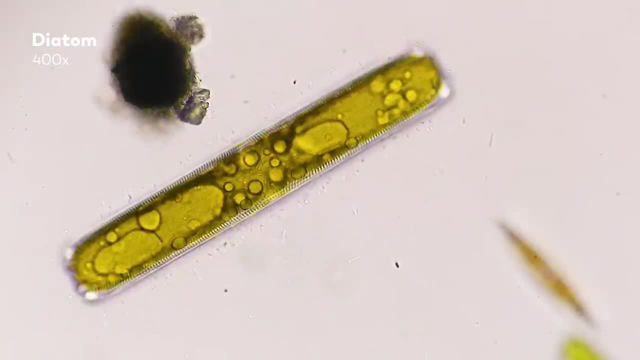 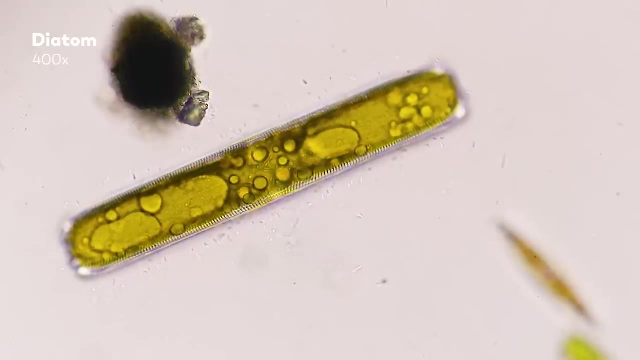 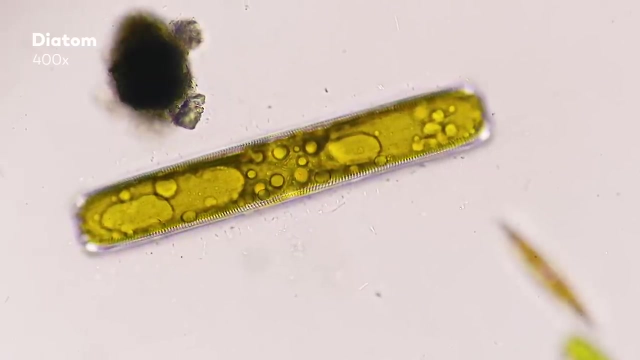 And if you are, we hope we can surprise you. Those are oil droplets And they store energy for the diatom when they might be having trouble finding light or their usual nutrients. These little organisms are so good at creating this fatty oil that scientists have wondered. 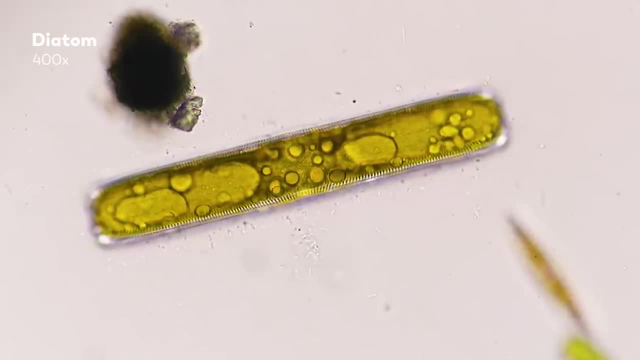 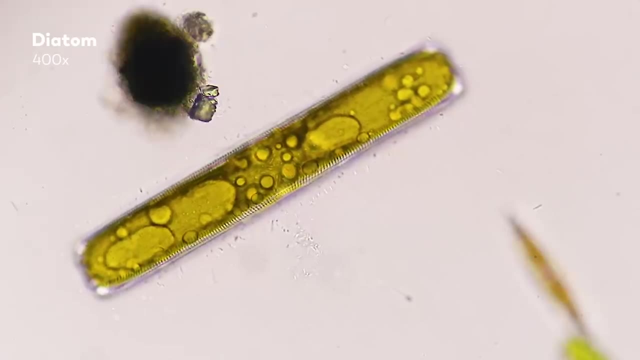 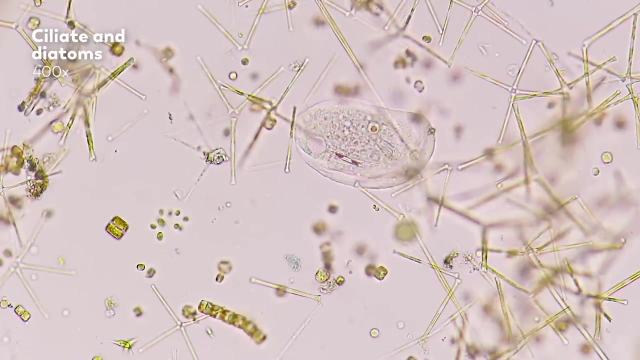 whether we might use diatoms as tiny factories that turn sunlight and carbon dioxide into fuel, not just for them but for our future airplanes. It might be a little complicated, tempting to think of these cells: just as little, microscopic jewels, just something nice to. 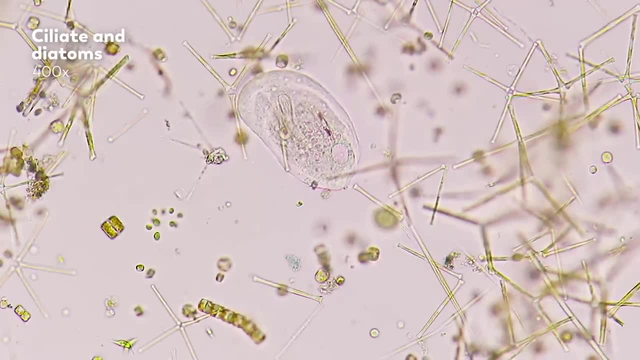 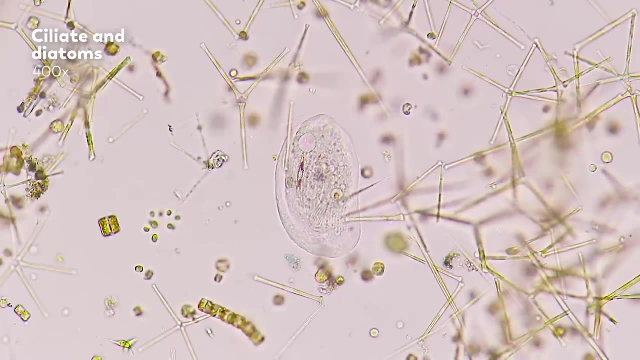 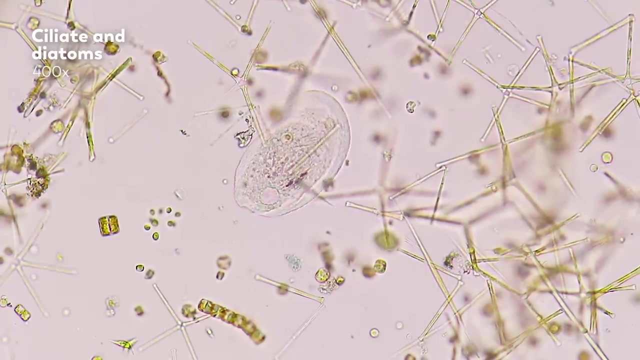 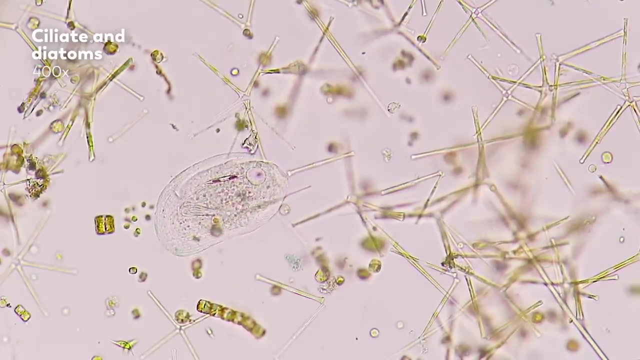 look at, But they also have a huge impact on our world. Of all of the photosynthesis being done on Earth, around one-fifth is done by diatoms, which puts them on par with all rainforests on Earth combined, And it means that we owe a great deal to these microorganisms, and not just our oxygen.